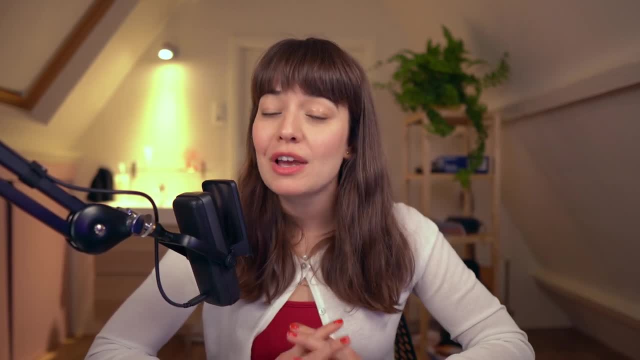 Training your machine learning model with the data that you have is not enough. You also have to evaluate it to understand if it needs to be improved or if it's going to perform well in the real world or not, And to do that we use evaluation metrics Depending on the type of 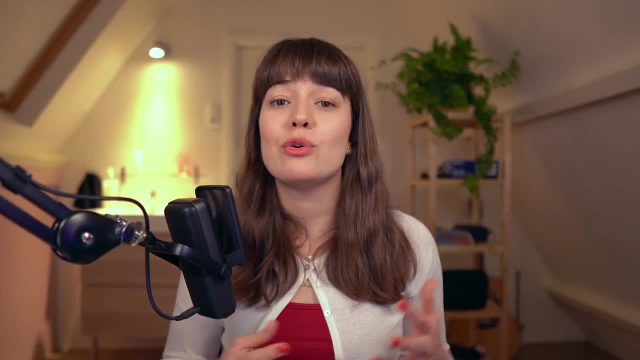 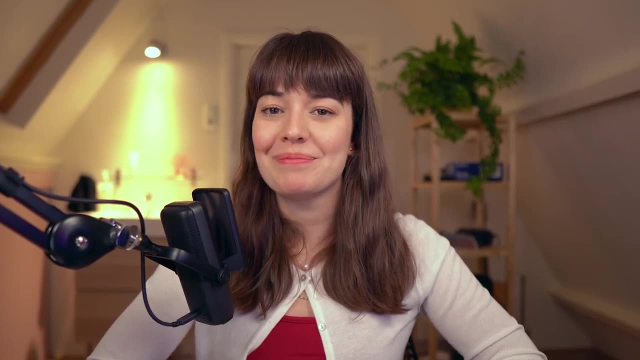 problem that you have. the kind of evaluation metric you're going to use is going to be different. So in this video, we will learn about evaluation metrics, what they mean and in which cases to use them. This video is brought to you by Assembly AI. Assembly AI is a company that is 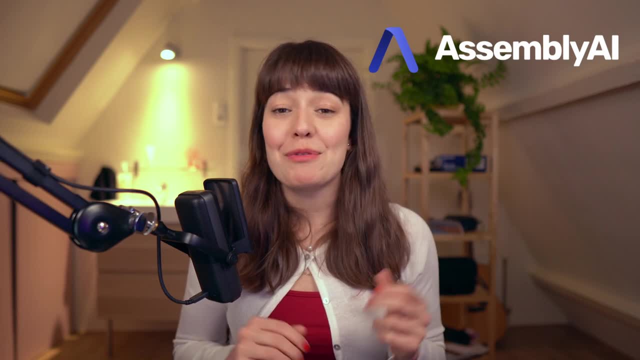 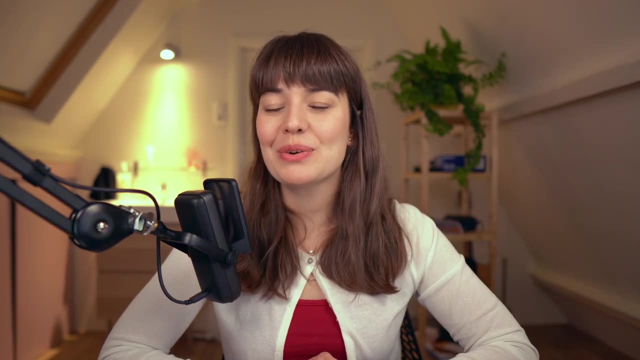 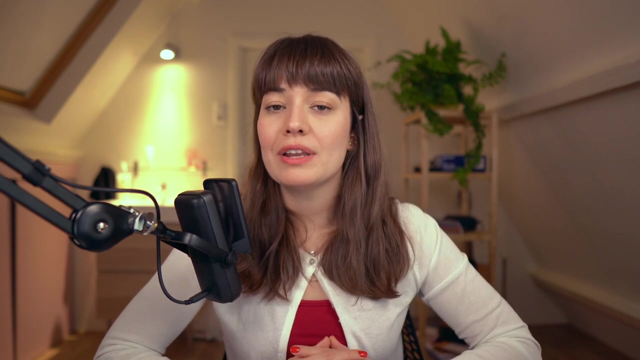 making a state-of-the-art speech-to-text API. If you want to try it out for free, go and grab your free API token using the link in the description. All right, let's get started. So let's first take a look at evaluation metrics that we use for classification tasks. The most popular one is: 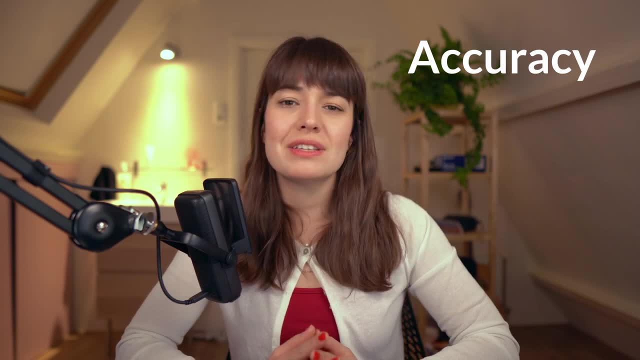 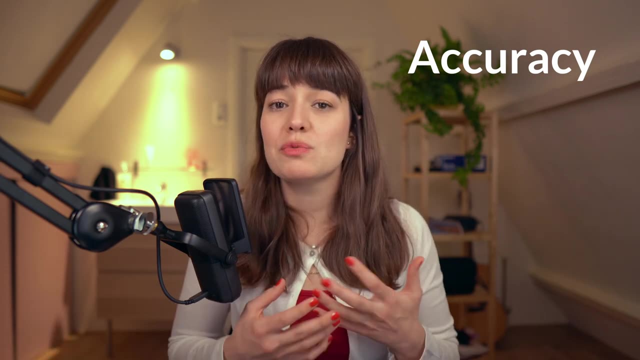 accuracy, and the reason that it's being used so much is because it's a very simple metric, It's very easy to understand and it's also very easy to compare different models with each other, because it's just one number that you need to look at. 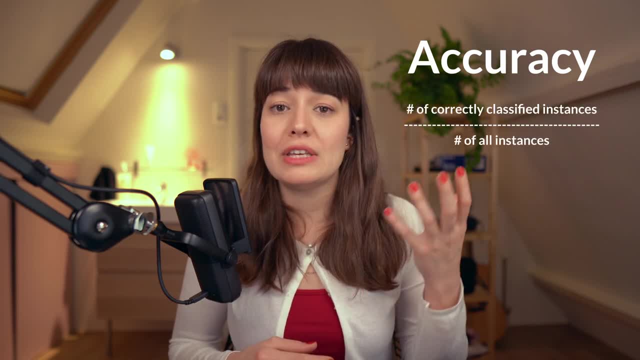 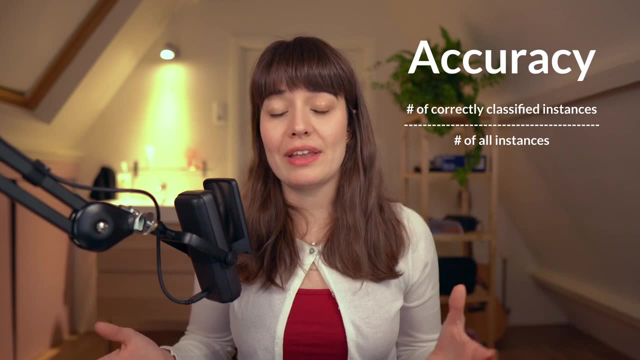 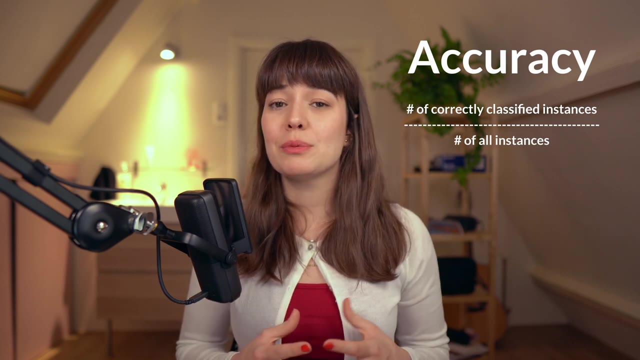 Accuracy is basically how many of the instances that you got right divided by the total number of instances that you have. Even though it's simple and very popular at the same time, it might not always be the best thing for you to use, because accuracy simplifies things a little bit too much. 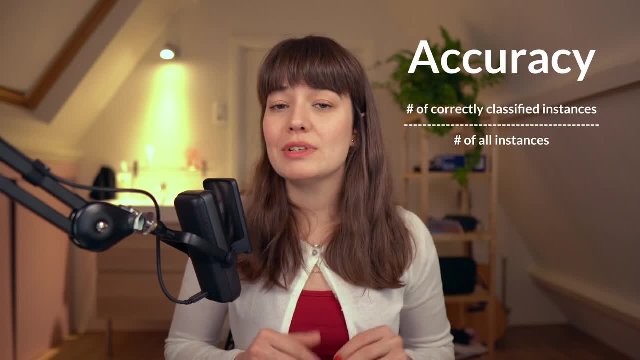 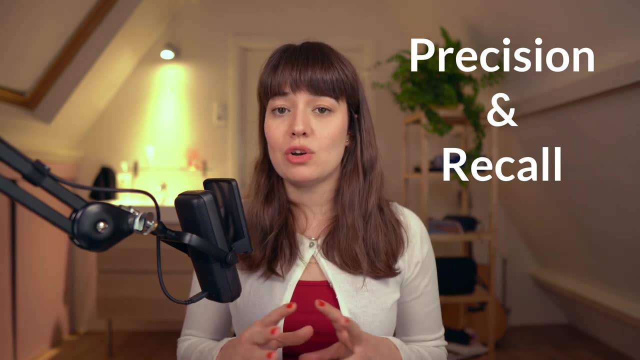 and that's why you might need to look into things that are a little bit more detailed, like precision and recall. So precision and recall are classification metrics, but they are mainly defined on true, positive and false positive. This is where you will find out why accuracy is important, and 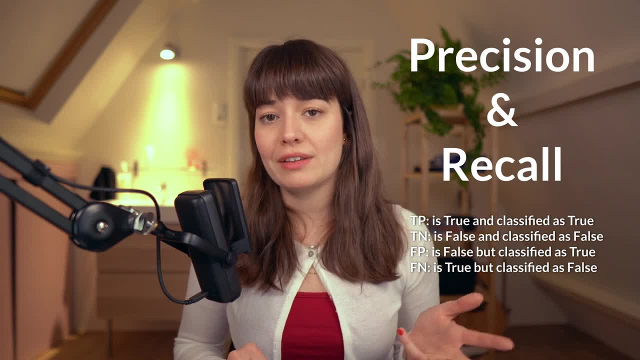 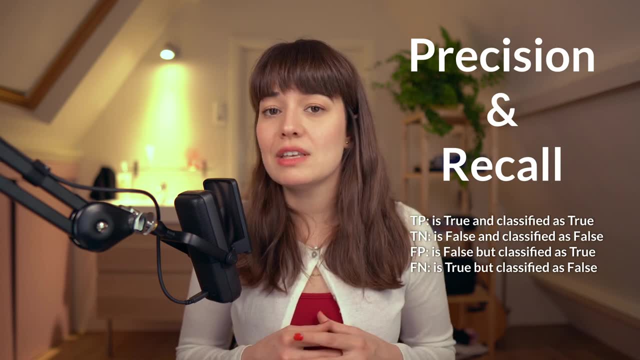 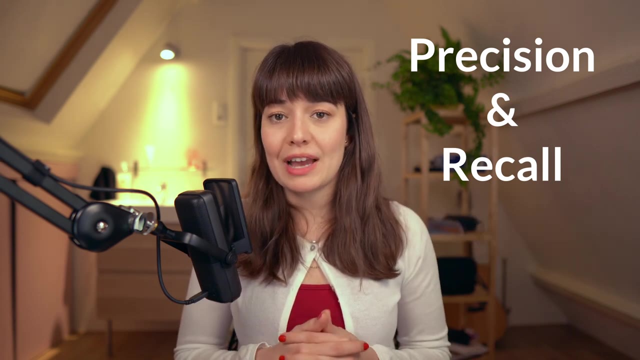 true positives, true negatives, false positives and false negatives. But this implies that the problem needs to be a binary classification of tagging the instances either with 0 or 1 or true or false. But you can actually use precision and recall for some other classification tasks. 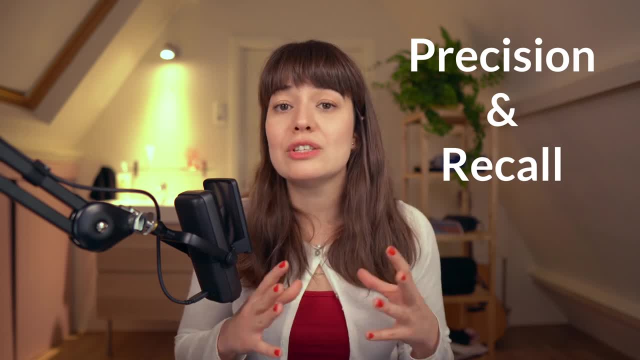 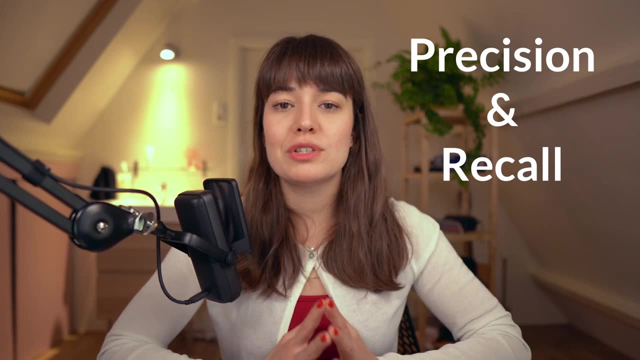 too. You don't only have to have true or false or only two different classes. So we will look into what we would do if we are not dealing with a binary classification task. but let's first define precision and recall thinking that we're doing a binary classification task. Precision is the 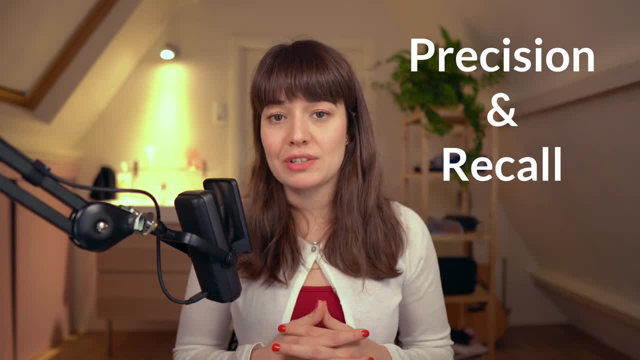 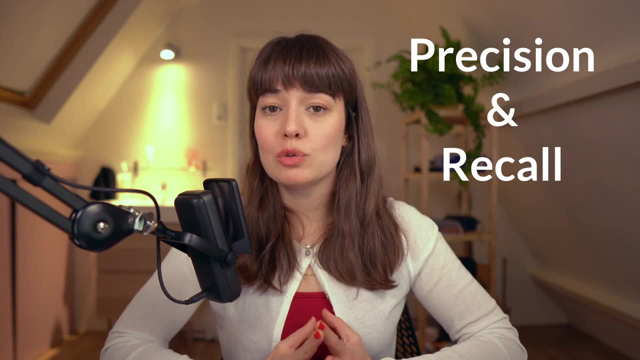 actually use precision and recall for some other classification tasks too. You don't only have to have true or false or only two different classes. So we will look into what we would do if we are not dealing with the binary classification task. But let's first define precision and recall. 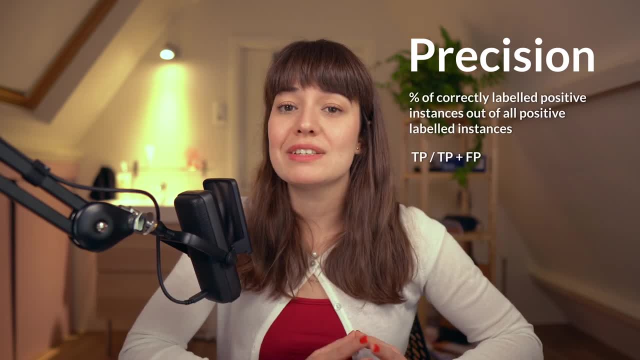 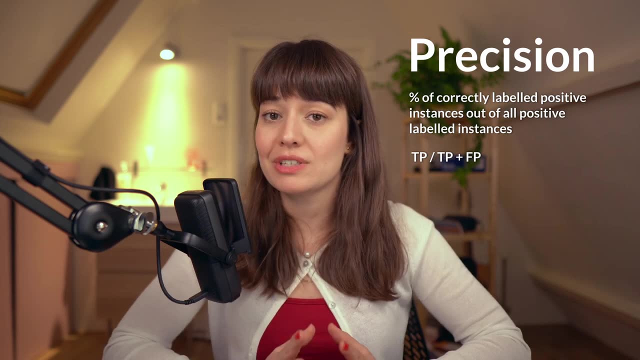 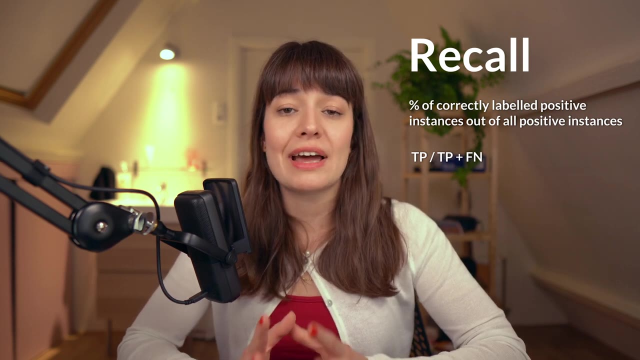 thinking that we're doing a binary classification task. Precision is the percentage of correctly labeled positive instances out of all the instances that were labeled as positive, Whereas recall is the percentage of correctly labeled positive instances out of all the instances that are actually positive. So, basically, precision tells us out of everything that I labeled as. 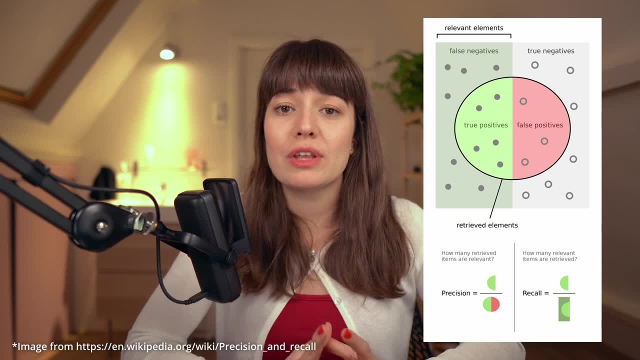 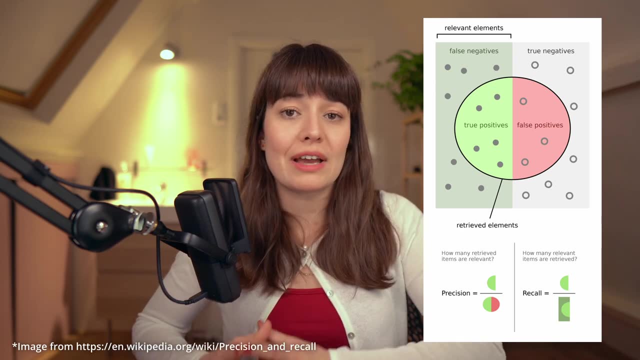 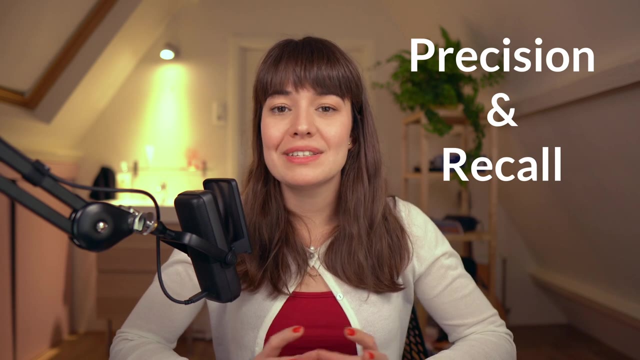 positive or as one of the classes, how many of them were actually belonging to that class, Whereas recall tells us, out of everything that belonged to that class, or you can say out of everything that was positive, how many of them I was able to capture, Because they are slightly. 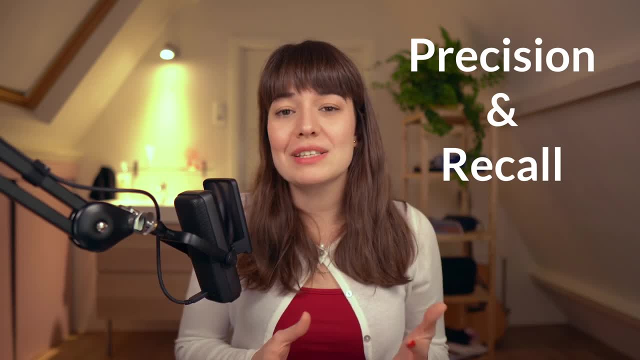 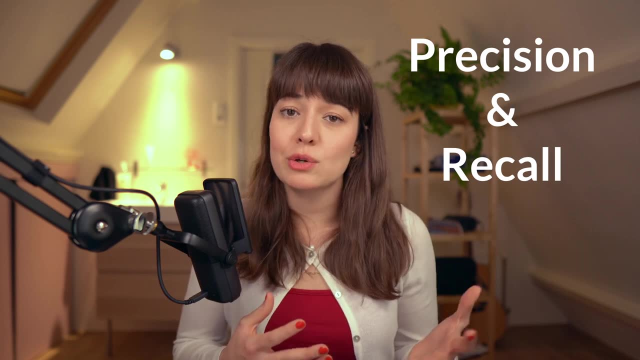 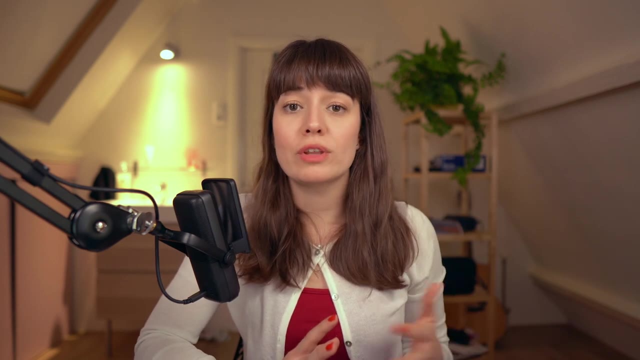 different. they give us different perspectives to the same model and that's why, most of the time, they are used together And by looking at the precision and recall values, it's easier to understand what's going wrong in the model And to also improve it. As I mentioned, sometimes your classification problem might have more than 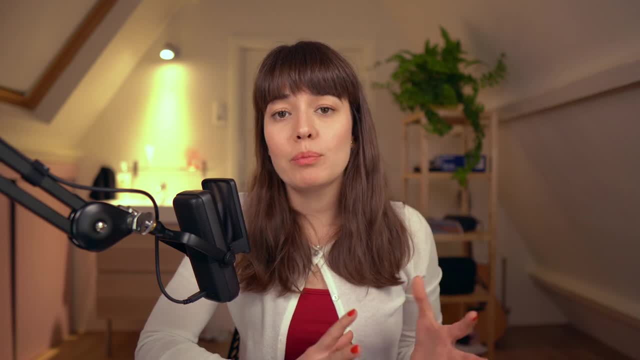 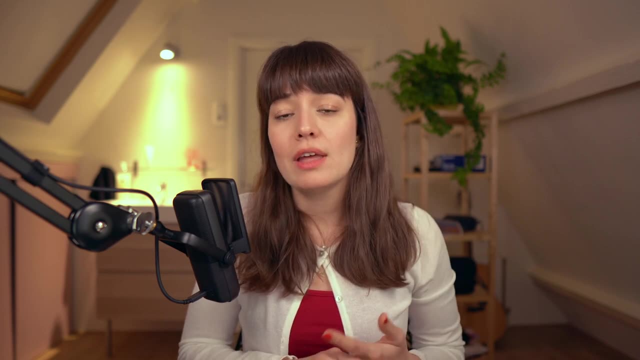 one class that you want to classify things into. At that point, you might want to use different approaches to your either accuracy, precision or recall. whatever you're calculating, There are a bunch of different ways to do that. One of the ways to do is to just calculate all of these values for 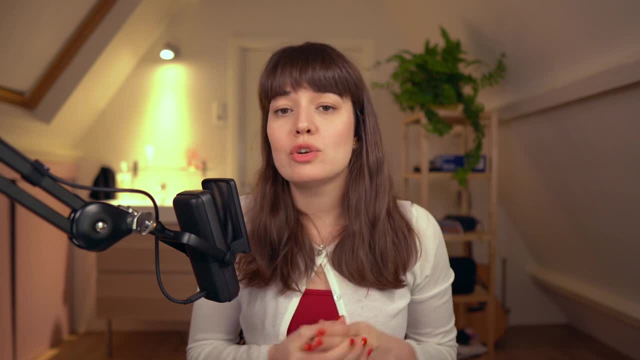 all of the different classes and then take their average. You can also weigh one of the classes or the others based on how important they are to you, And then you can also weigh one of the classes or the others based on how important they are to you, And then you can also weigh one of the classes or 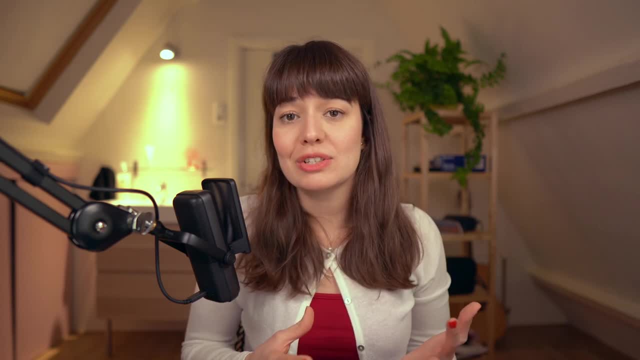 the others based on how important they are to you, And then you can also weigh one of the classes or the others based on how important they are to get correctly, And then again take the average, The average. it is important to decide on the correct way to calculate accuracy, precision and 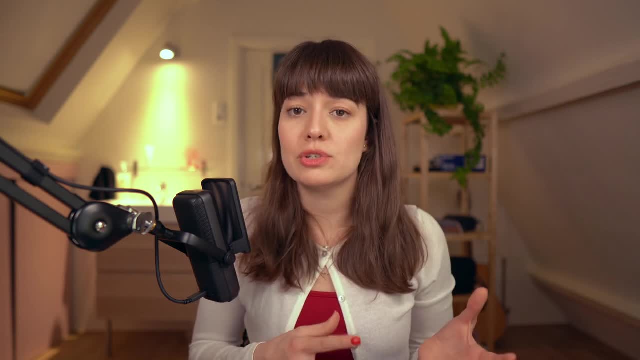 we'd call a test experience, if you want to. The pass base is basically that you decide whether you want to show your answer the first time or the second time. You will learn after it's done, So before you go forward with some of the more difficult ones, obviously it's morning, so why there's someone that isn't learning anything yet. However, but the most important thing, before you go forward with those ones, make sure that you check a documentation of the type of three out of 50 census data issues, so you can read them all and find what's not. 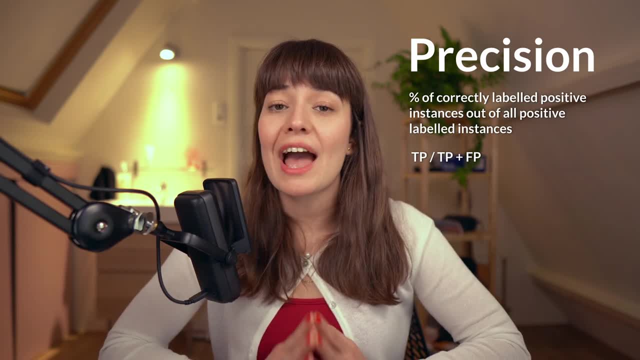 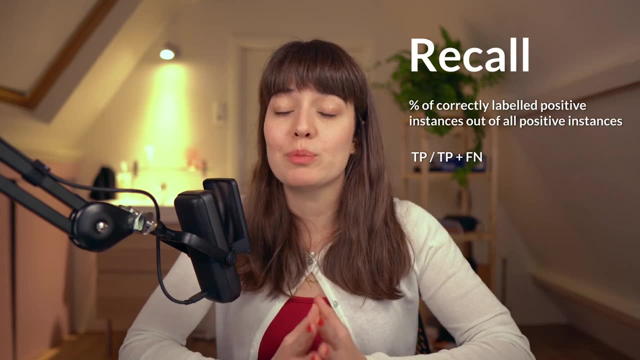 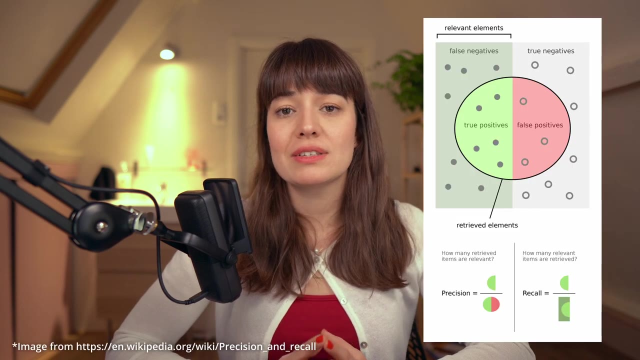 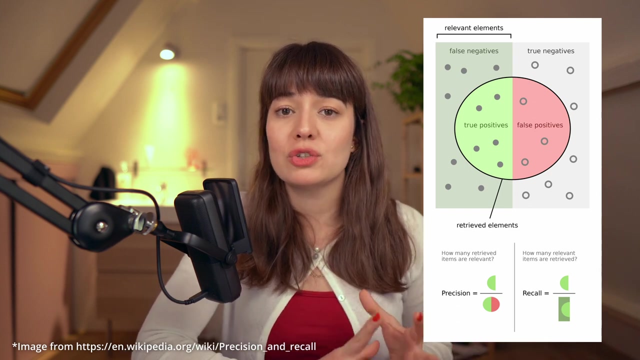 percentage of correctly labeled positive instances out of all the instances that were labeled as positive, Whereas recall is the percentage of correctly labeled positive instances out of all the instances that are actually positive. So, basically, precision tells us, out of everything that I labeled as positive or as one of the classes, how many of them were actually. 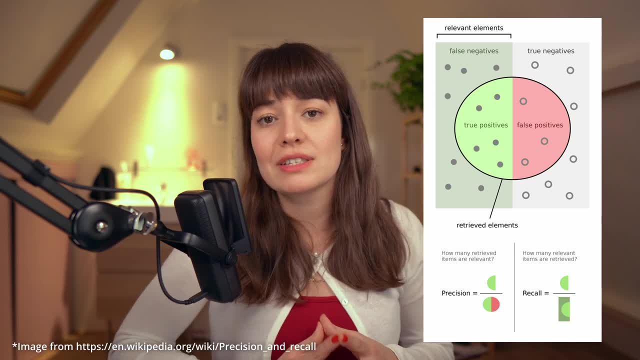 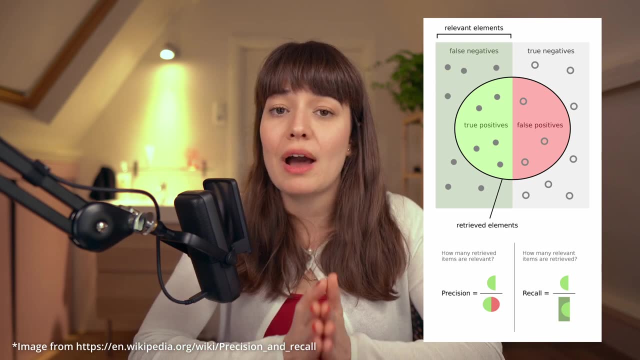 believable, So we can use precision and recall to define precision and recall, thinking that we're belonging to that class, Whereas recalls tells us, out of everything that belonged to that class, or you can say, out of everything that was positive, how many of them I was able to capture, Because 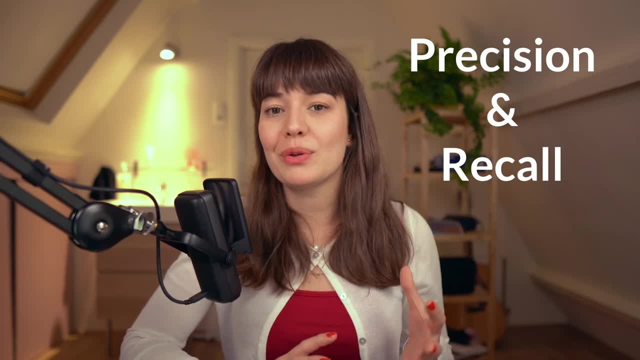 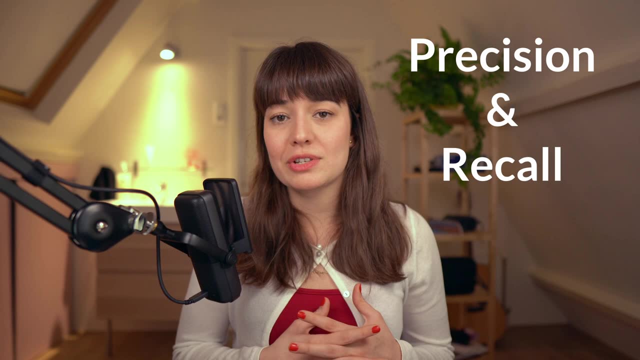 they are slightly different. they give us different perspectives to the same model And that's why, most of the time, they are used together And by looking at the precision and recall values, it's easier to understand what's going wrong in the model and to also improve it. As I mentioned, sometimes your 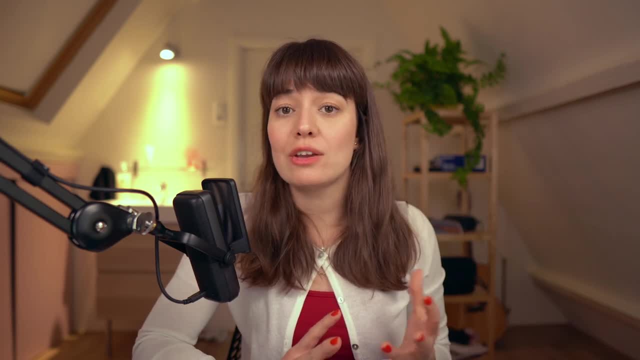 classification problem might be a little bit more difficult to understand than it is to understand what's going on in the model. So you might have more than one class that you want to classify things into. At that point you might want to use different approaches to your either accuracy. 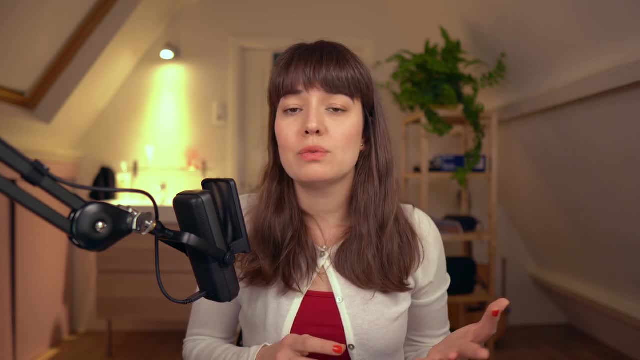 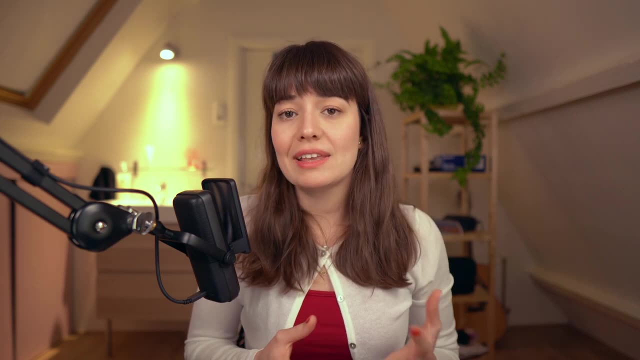 precision or recall whatever you're calculating. There are a bunch of different ways to do that. One of the ways to do is to just calculate all of these values for all of the different classes and then take their average. You can also weigh one of the classes or the others. 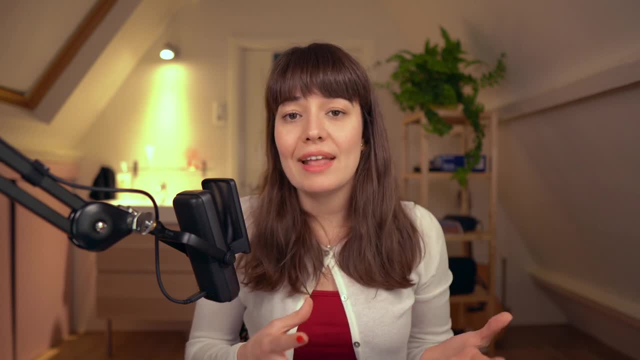 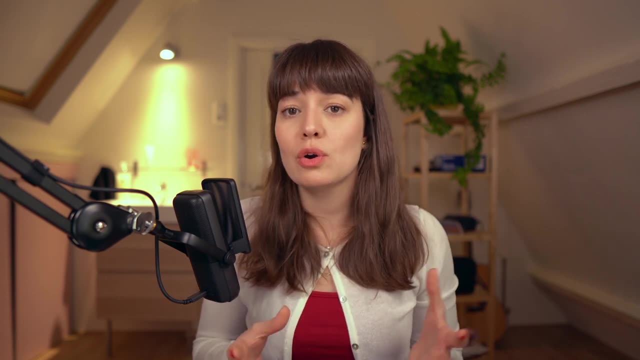 based on how important they are to get correctly And then again take the average. It is important to decide on the correct way to calculate accuracy, precision and recall based on the kind of problem that you have. So before you go forward with those ones, make sure that you check the documentation. 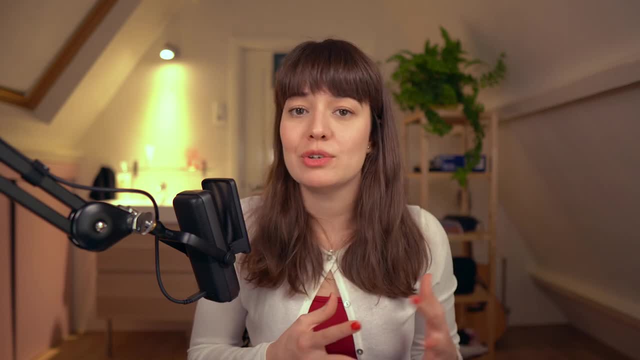 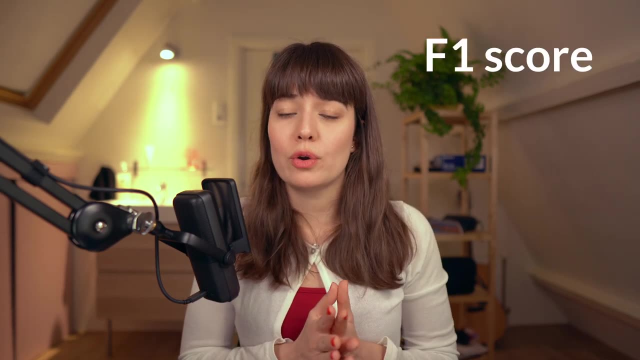 of the type of framework that you're using or the type of library that you're using, and to choose the correct one for your problem. Another thing that you can use is called the F1 score. It is a combination of precision and recall and it gives you only one number, So sometimes people 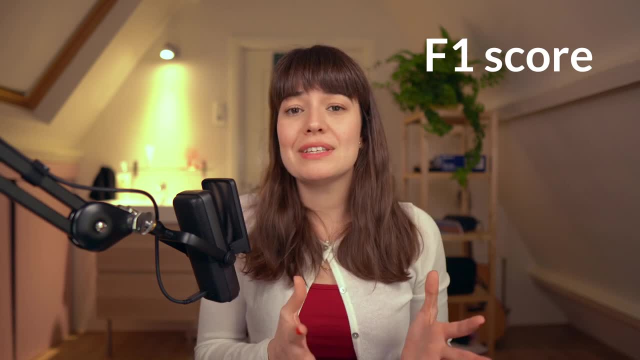 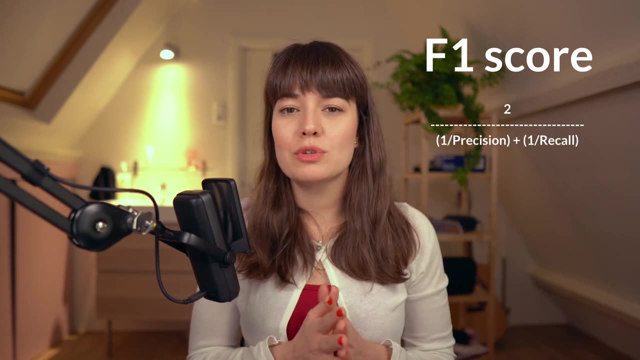 prefer to look at F1 score. F1 score is a number that you can use to calculate accuracy, precision and recall. F1 score is basically a harmonic mean of precision and recall and this is how it's calculated. But remember that F1 score is, most of the time, best used in combination with other. 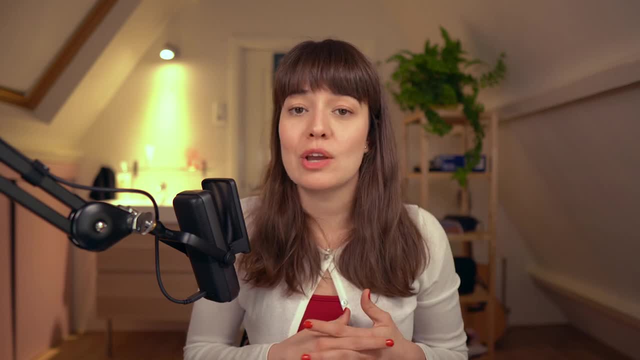 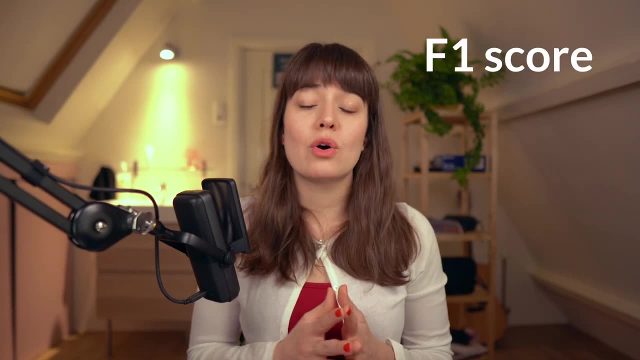 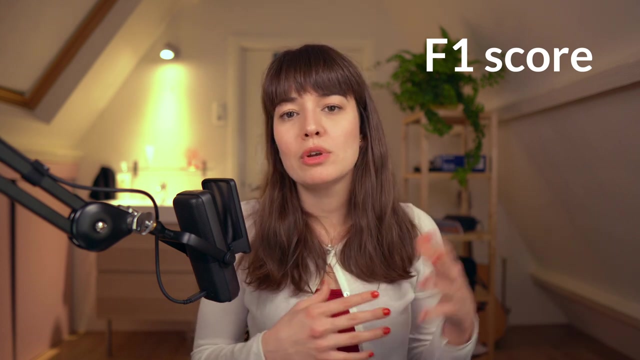 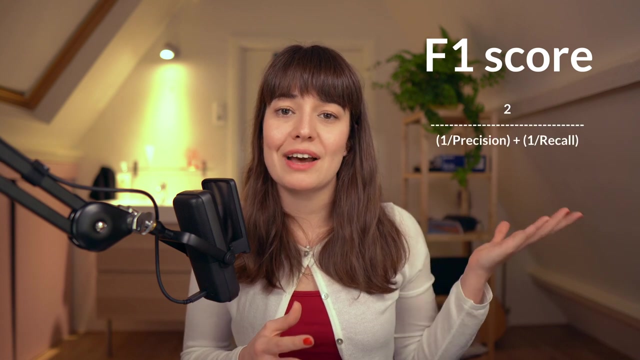 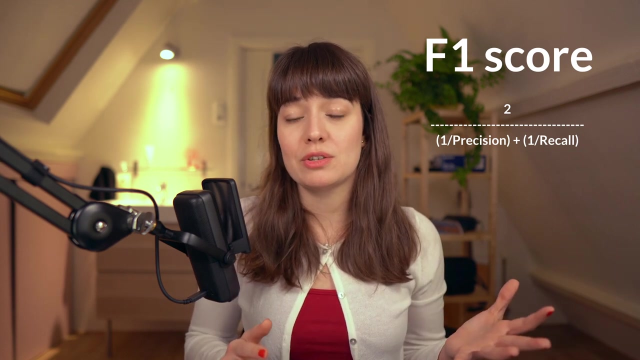 документ 80, only one number, So sometimes people prefer to look at F1 score. F1 score is basically a harmonic mean of precision and recall and this is how it's calculated. But remember that F1 score is most of the time best used in combination with other metrics, So, for example, the PR curve or the ROC. 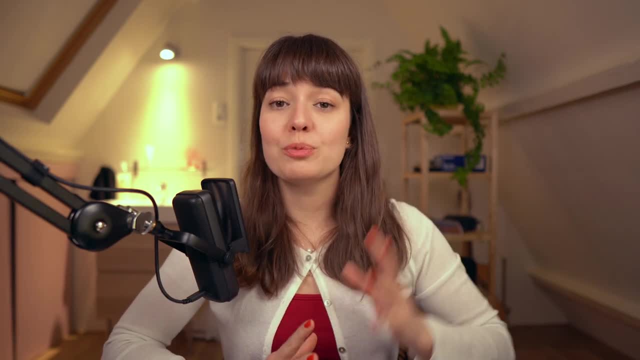 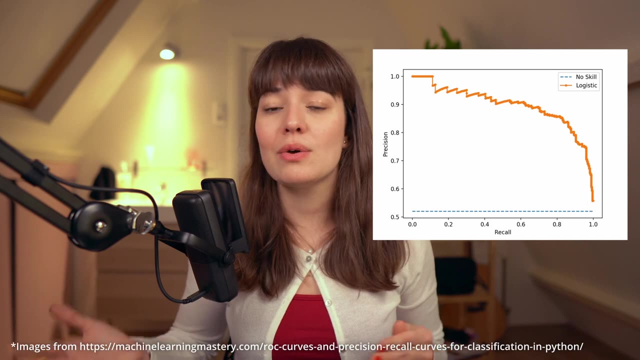 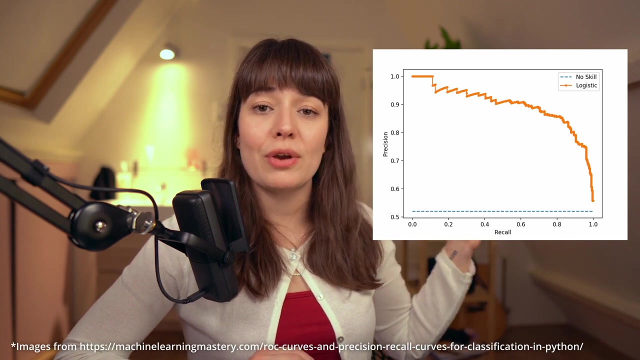 curve. So let's talk about them now. PR curve is called precision and recall curve. It's basically a comparison of what the recall is when precision has this value, and also vice versa. So in this example graph, for example, we would want the curve to be on the top right corner, because that's the 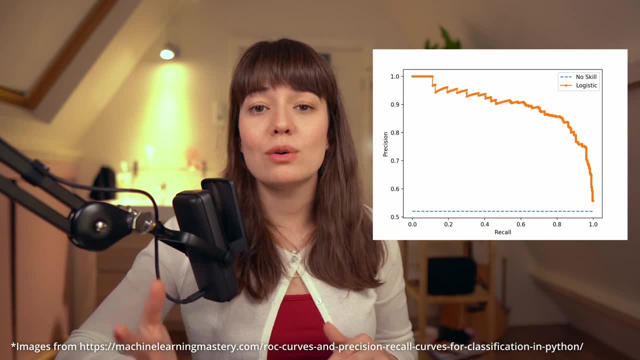 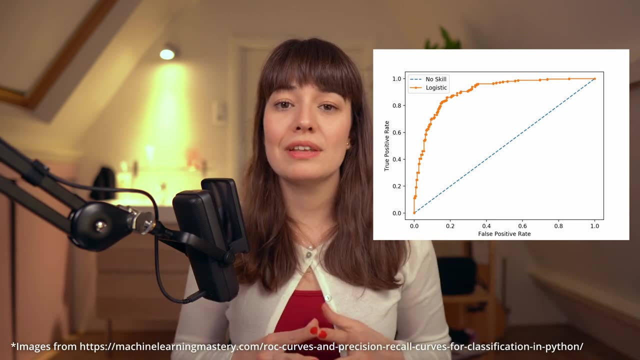 point where we have a high precision value and also a high recall value. ROC curve, on the other hand, is again very similar, but this time you are comparing the true positive rate to the false positive rate. By looking at these two different graphs, you can see that the precision is very similar to the recall curve. So if you look at the 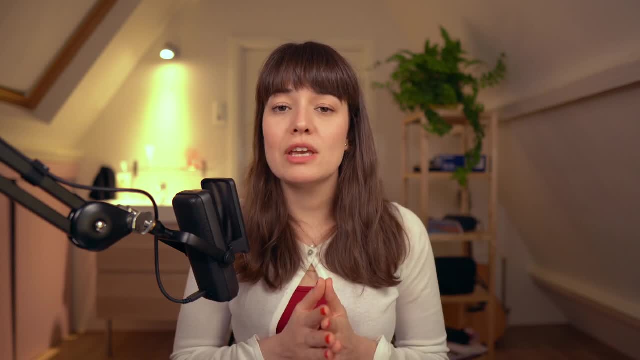 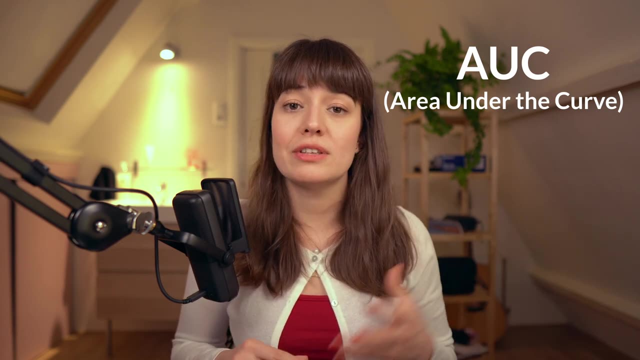 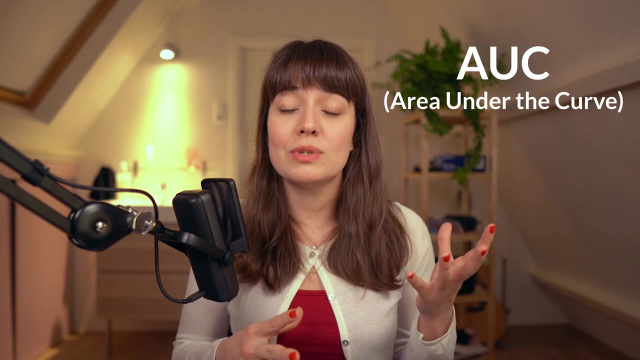 you can understand how your model is performing better. and sometimes you would hear people use the word AUC area under the curve, and sometimes they calculate this using the PR curve and sometimes they calculate this using the ROC curve. But either way, you want this AUC number to be as. 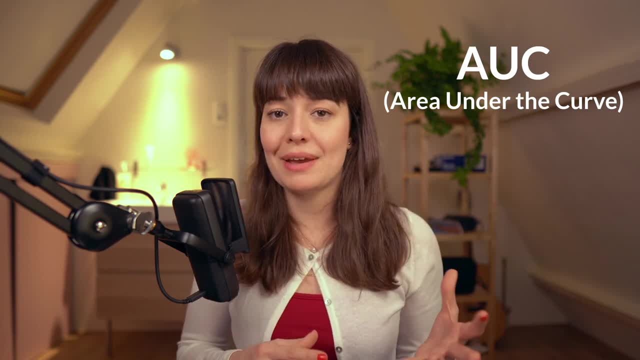 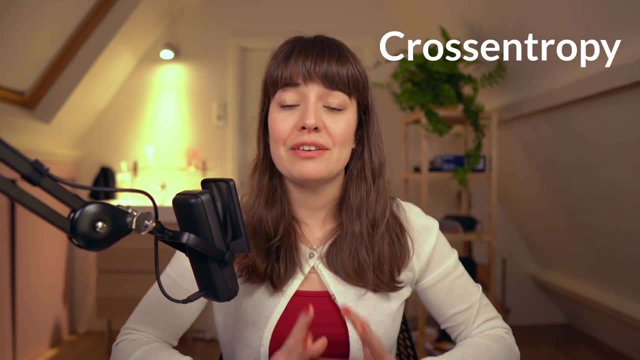 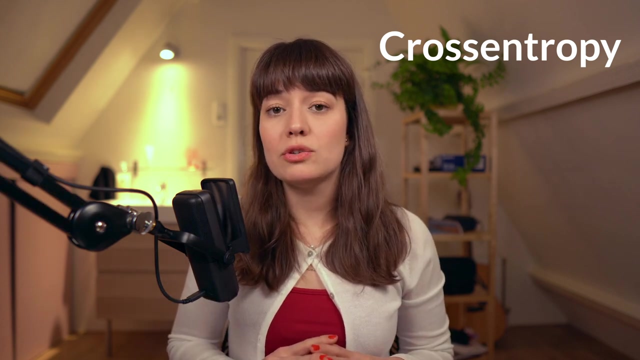 high as possible, because then you know your model is performing the best. And lastly, for classification tasks, we have cross entropy. Cross entropy basically calculates the difference or the distance between two probability distributions. Depending on the kind of problem that you have, you might need to use binary cross entropy, categorical cross entropy or sparse categorical. 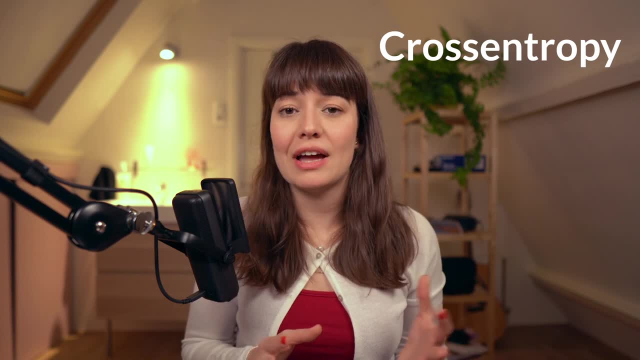 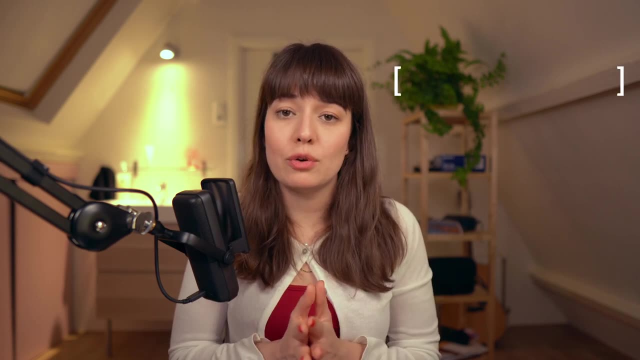 cross entropy. But these are different implementations that you can find easily, for example in the Keras library. For example, let's say you have a one hot encoded classification for your model and that goes 0, 1, 0. So your model belongs to your instance, belongs to the second. 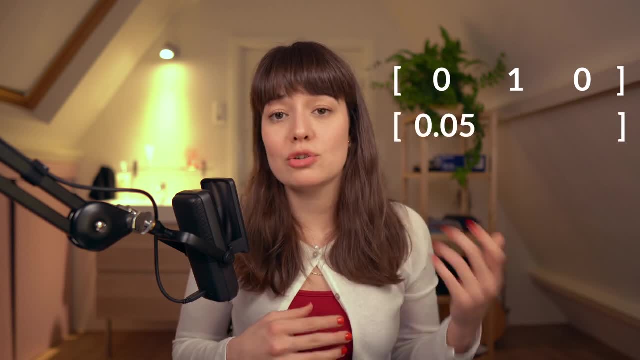 class, and if your outcome from your model is 0, 1, 0, then your instance belongs to the second class. If your model is, let's say, 0.5, 0.95 and then 0.0, that means that your model has classified it with. 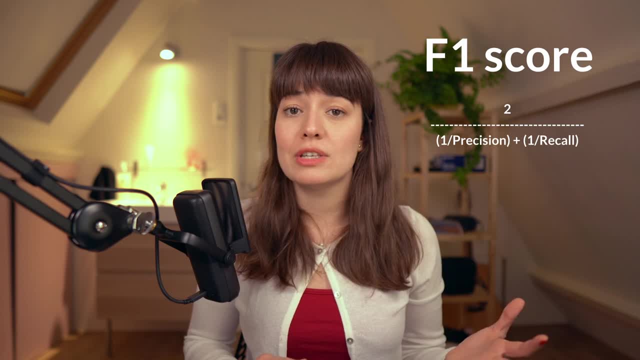 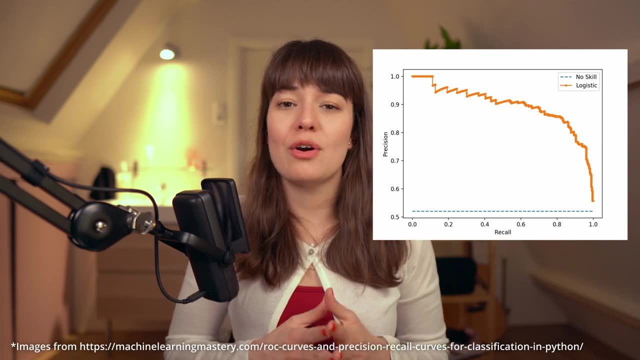 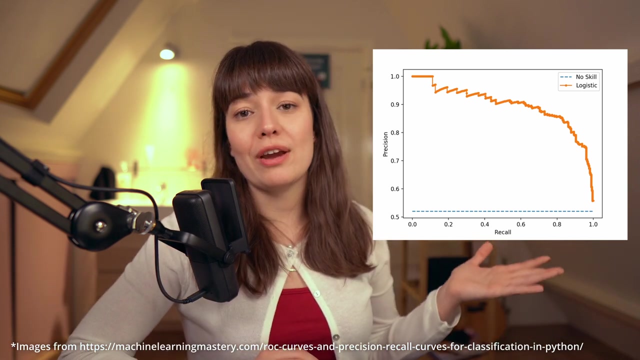 metrics, So, for example, the PR curve or the ROC curve. So let's talk about them now. PR curve is called precision and recall curve. It's basically a comparison of what the recall is when precision has this value and also vice versa. So in this example graph, for example, we would want the 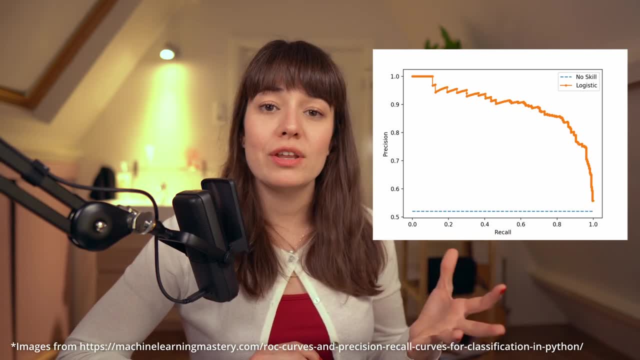 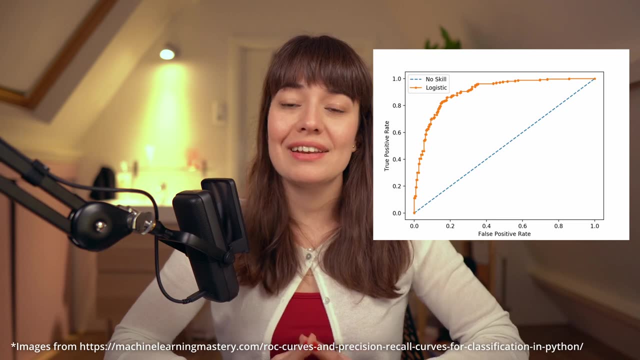 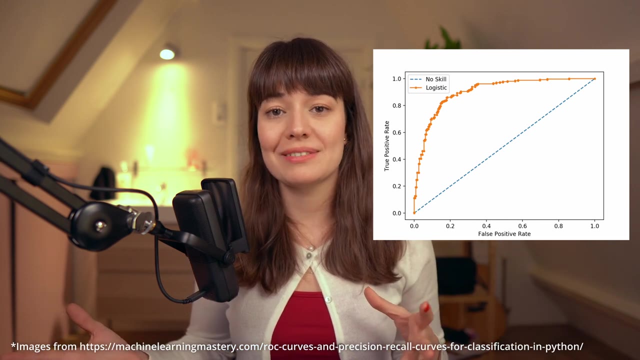 curve to be on the top right corner, because that's the point where we have a high precision value and also a high recall value. ROC curve, on the other hand, is again very similar, but this time you are comparing the true positive rate to the false positive rate. By looking at these two, 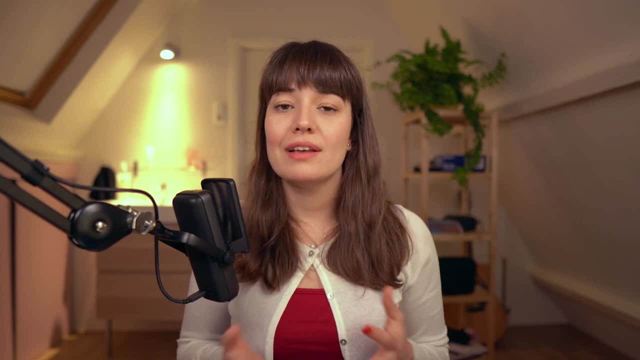 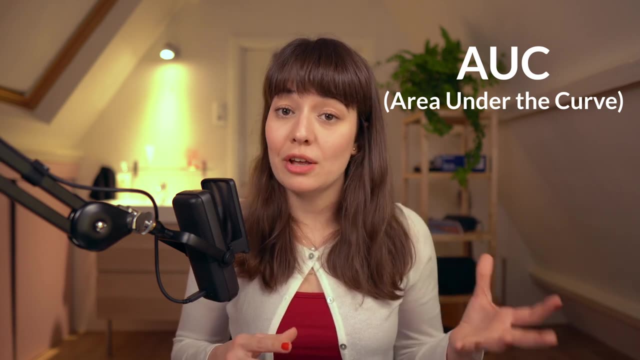 different graphs, you can understand how your model is performing better. and sometimes you would hear people use the word AUC, area under the curve, and sometimes they calculate this using the PR curve and sometimes they calculate this using the ROC curve. But either way you want. 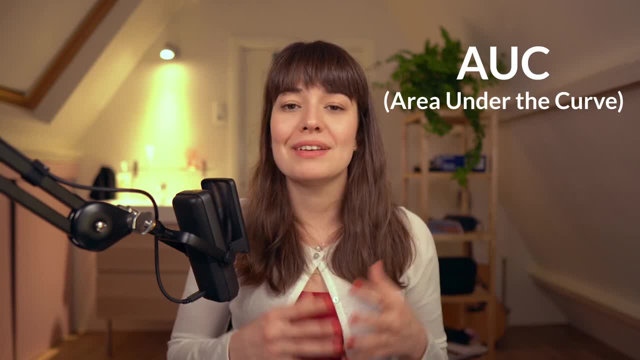 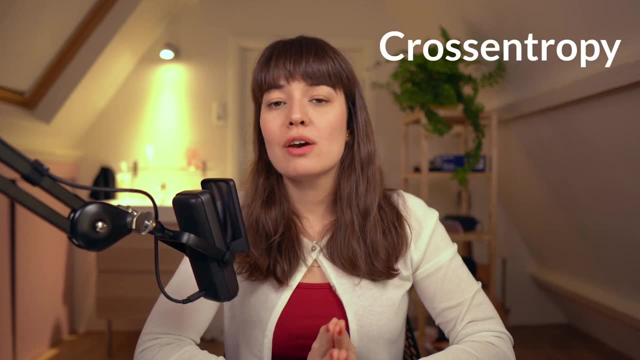 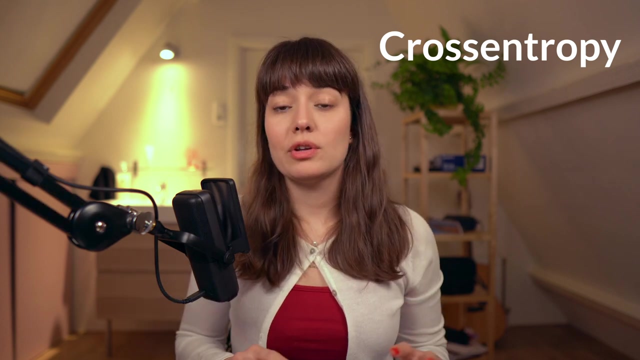 this AUC number to be as high as possible, because then you know your model is performing the best. And lastly, for classification tasks we have cross entropy. Cross entropy basically calculates the difference or the distance between two probability distributions, Depending on the 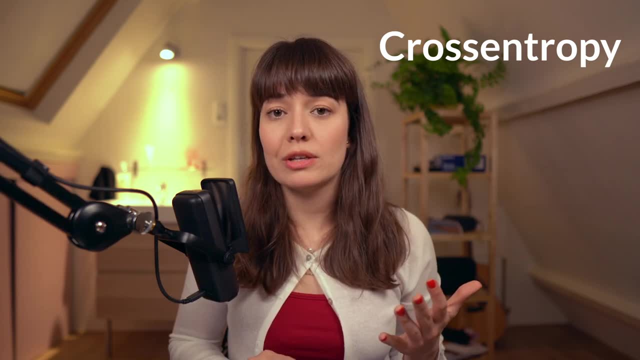 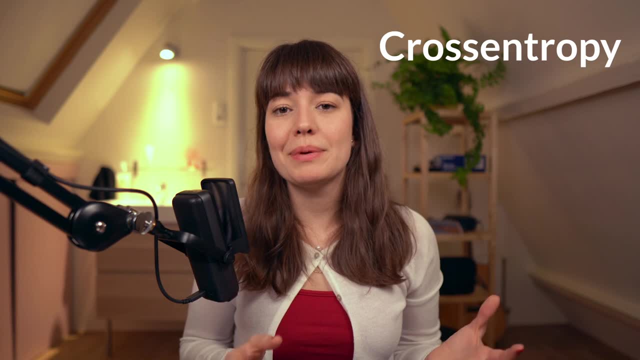 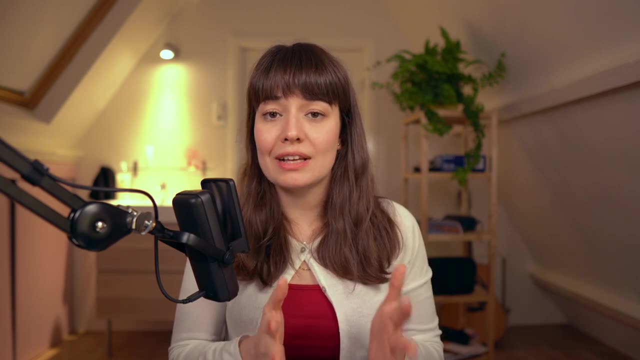 where you have a problem. where you have a problem where you have a problem- categorical cross entropy. But these are different implementations that you can find easily, for example, in the Keras library. For example, let's say you have a one-hot encoded classification. 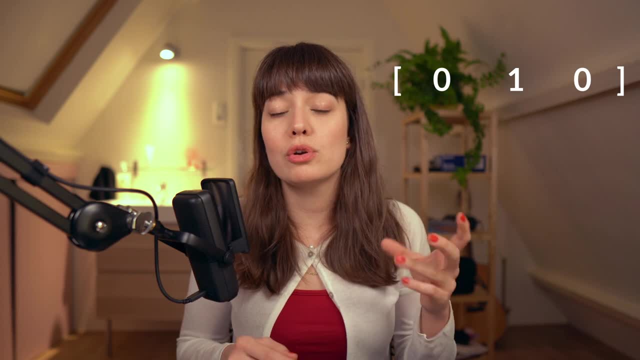 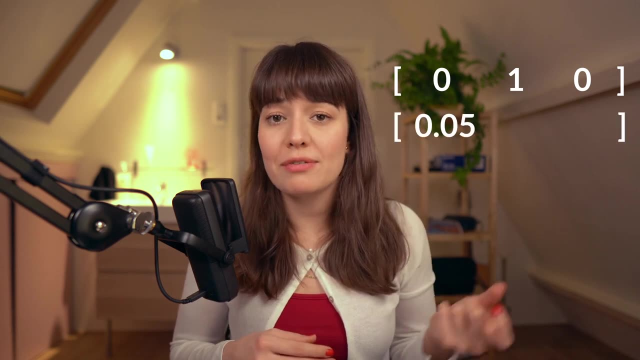 for your model, and that goes 0,, 1,, 0. So your model belongs, your instance belongs, to the second class, And if your outcome from your model is, let's say, 0.5,, 0.95, and then 0.0,, that means 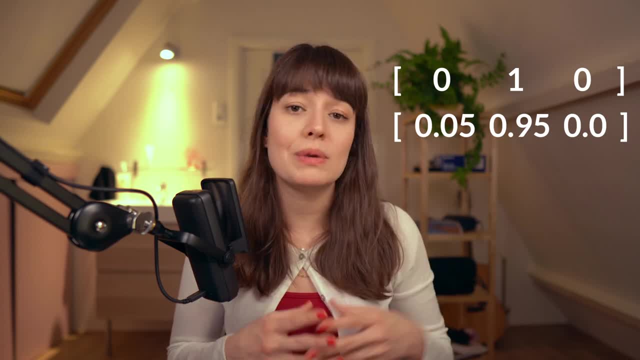 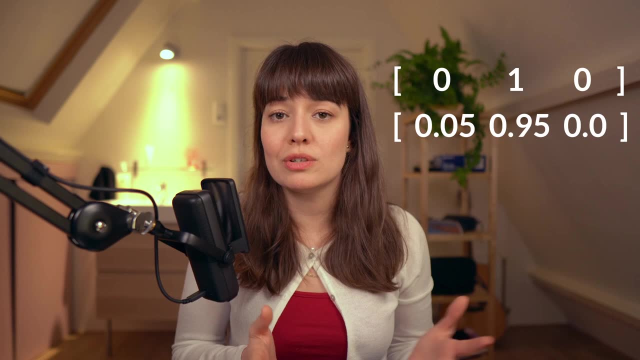 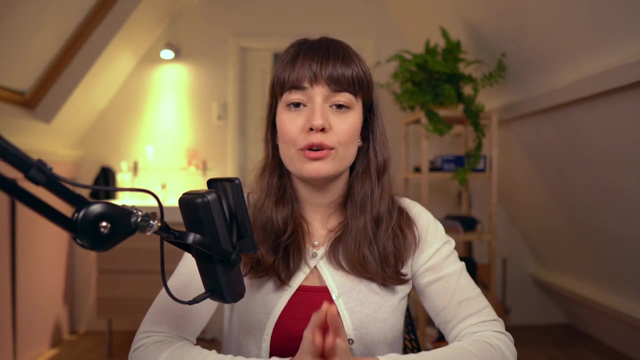 that your model has classified it with really high confidence to be the second class, But not fully. So that's why calculating the distance or the difference between these two distributions, is important to understand how accurate your model is. So let's talk about regression evaluation metrics. The first and the simplest one is called mean absolute error And, as 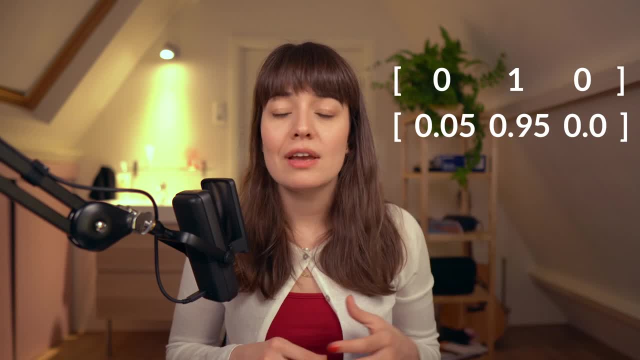 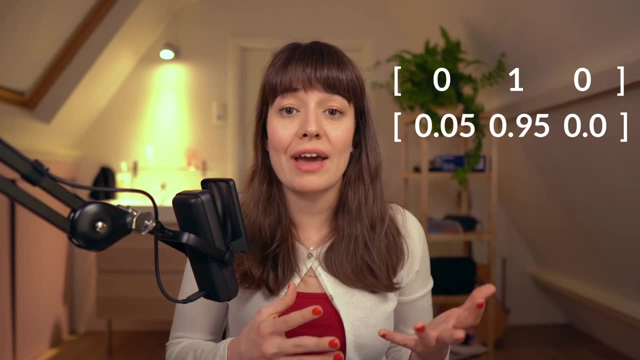 really high confidence to be the second class, but not fully. So that's why calculating the distance or the difference between these two distributions is important to understand how accurate your model is. So let's talk about regression evaluation metrics. The first and the simplest one is called 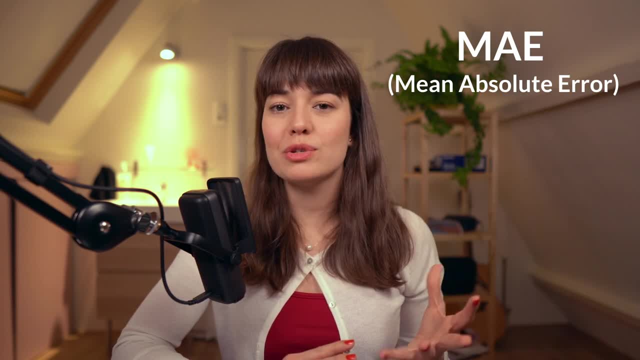 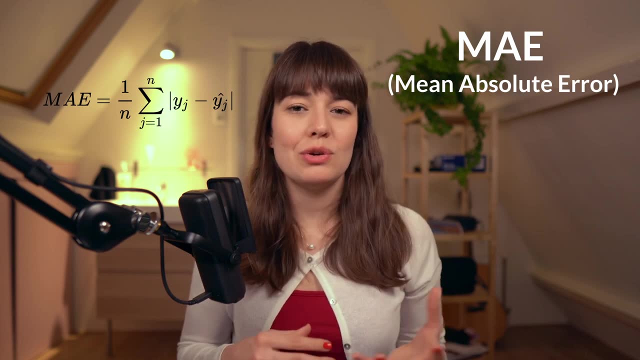 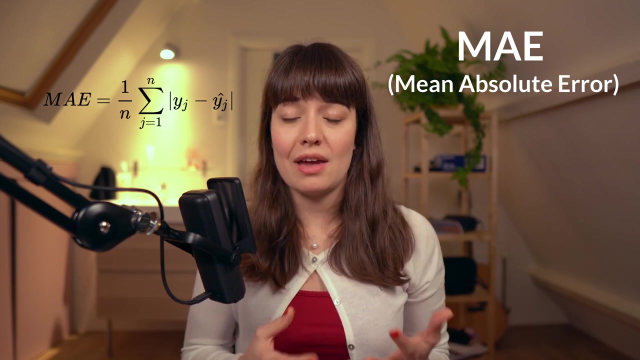 mean absolute error and, as you can understand from the name, also mean absolute error is basically sum of all the errors but their absolute values. Because if you do not take their absolute values, the minuses, the negative values might just cancel out the positive values and you might get an error or the mean error that actually looks very small. That's why, first you 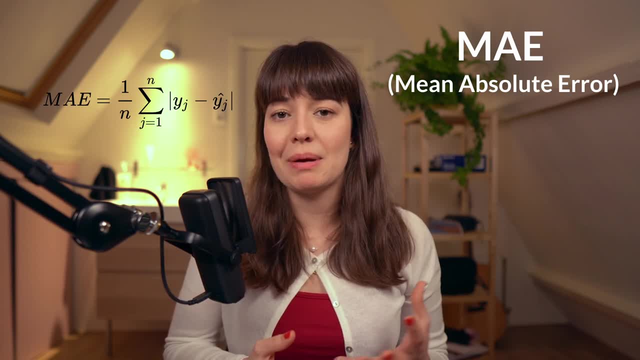 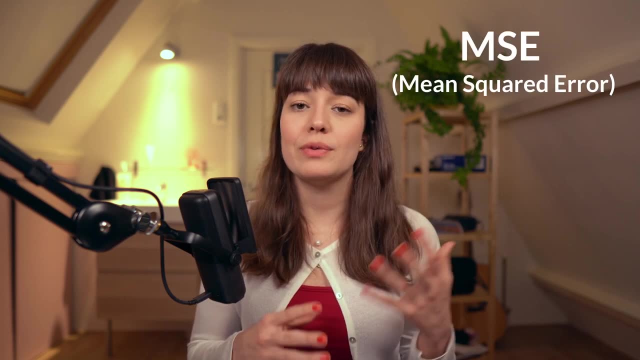 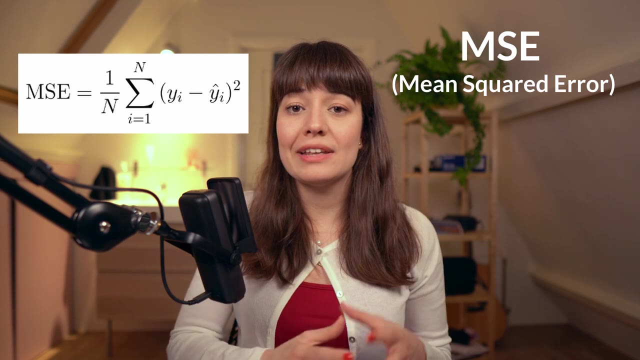 need to take all the absolute values of your errors and then sum them up together and take their mean. Another way to calculate the error for regression problems is called mean squared error, and the way you calculate it is basically taking the square of all the errors and then taking their mean. By doing that, you are letting the greater error 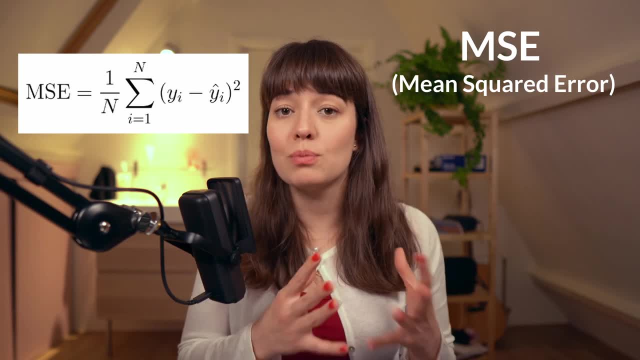 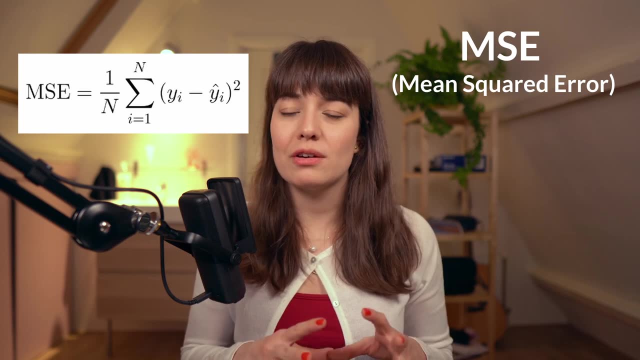 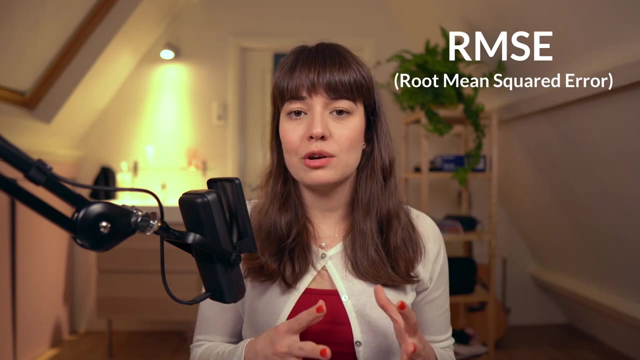 values to impact this mean squared error value more by exaggerating their importance, by getting their square. But this value, sometimes, the mean squared error value, sometimes can be a bit hard to understand. That's why instead we use root mean squared error and that is calculated by again. 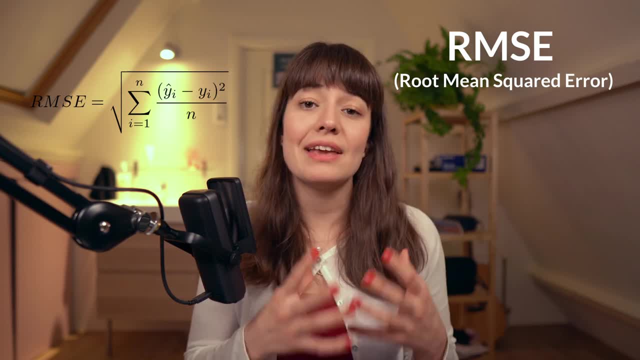 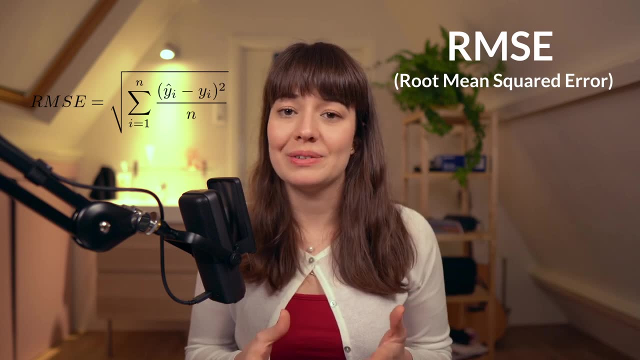 taking the square of all the errors, getting their mean and then getting the square root of this mean squared error. So if you take the square of all the errors and then taking their mean, this final value, So it's basically the square root of mean squared error. By doing that you're 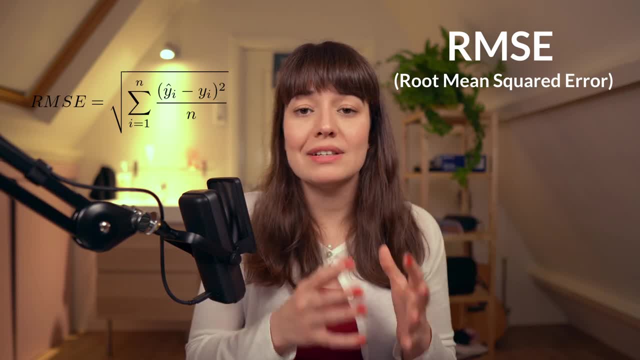 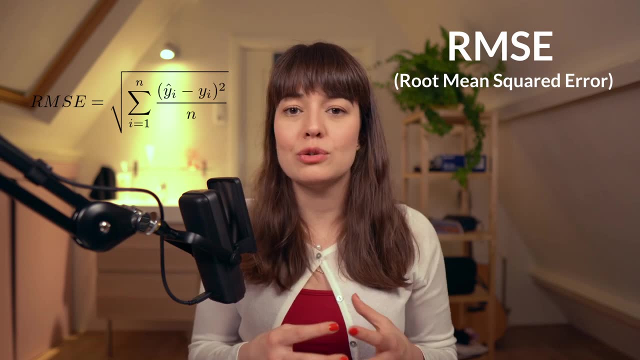 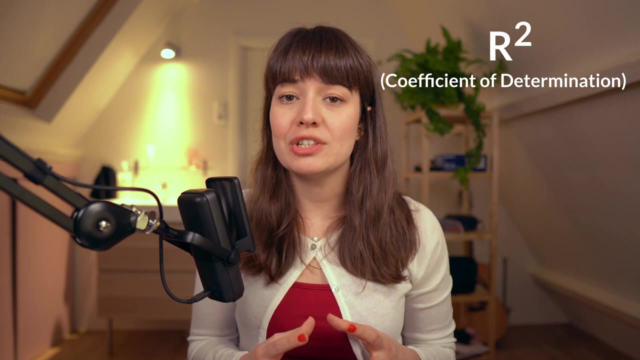 still exaggerating the importance of the greater error values, but still you're bringing it down to the scale of mean absolute error metric so that it's easier for you to compare these two metrics and understand what might be going wrong in your model. R squared or coefficient of determination. 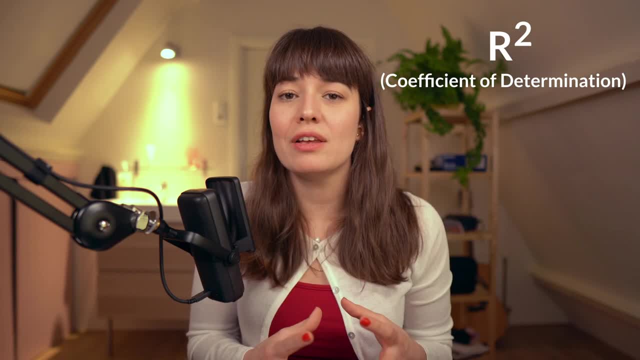 gives us a good measure of how well your model fits this data. So it's basically the measure of how well your model fits this data. So it's basically the measure of how well your model fits this data. So it's basically the measure of how well your model fits this data. So it's basically. 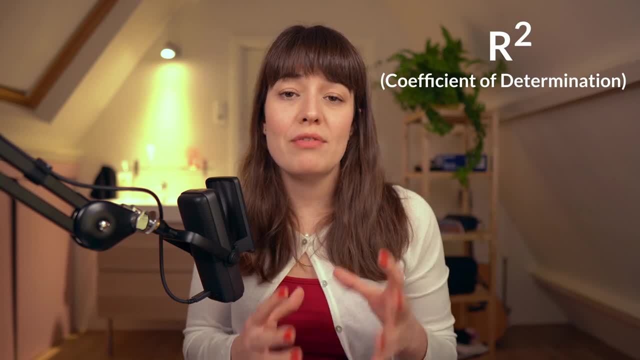 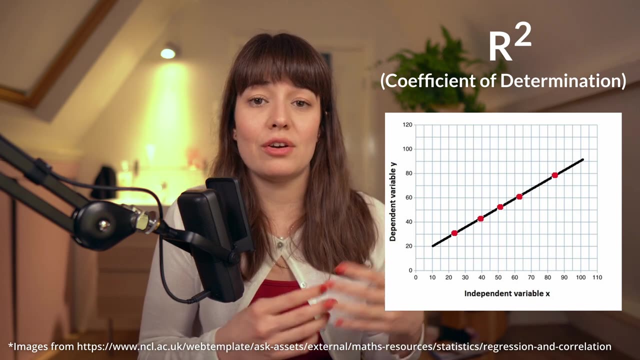 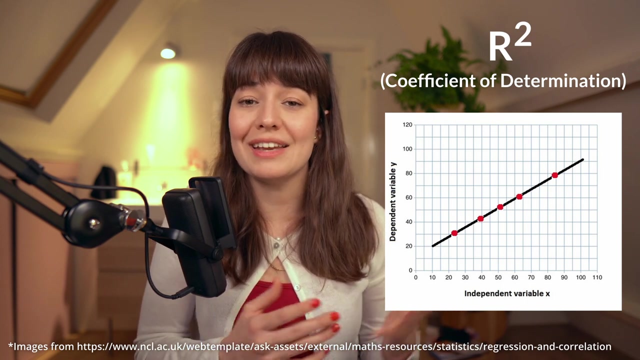 a metric of how much the real values vary from the curve that your model came up with. So if you look at this example, let's say this line is the curve that our model came up with and the dots are the values of the real values of the instances that we have in our data. So if all the values lie, 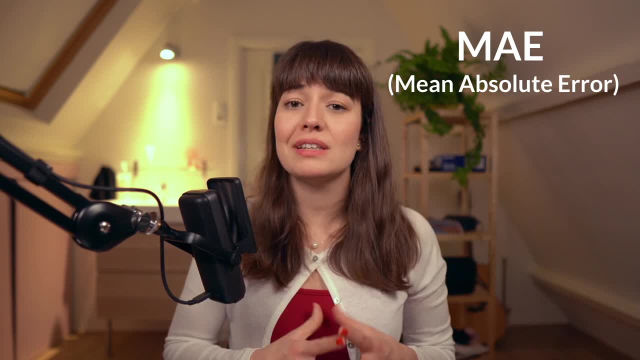 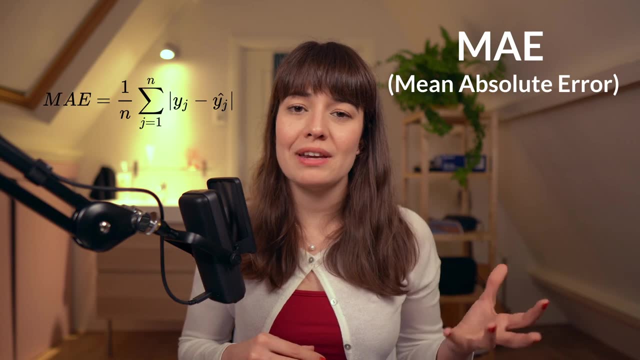 you can understand from the name, also mean absolute error is basically the sum of all the errors but their absolute values. Because if you do not take their absolute values, the minuses, the negative values might just cancel out the positive values and you might get an error or the mean error that. 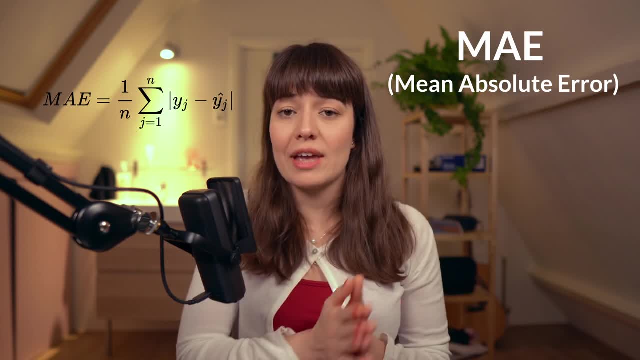 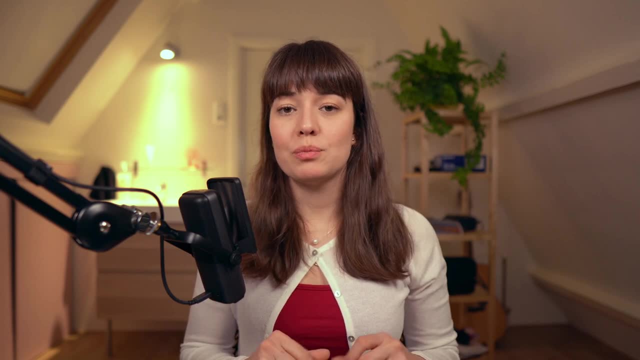 actually looks very small. That's why first you need to take all the absolute values of your errors and then sum them up together and take their mean. Another way to calculate the error for regression problems is called mean squared error, And the way you calculate it is basically taking. 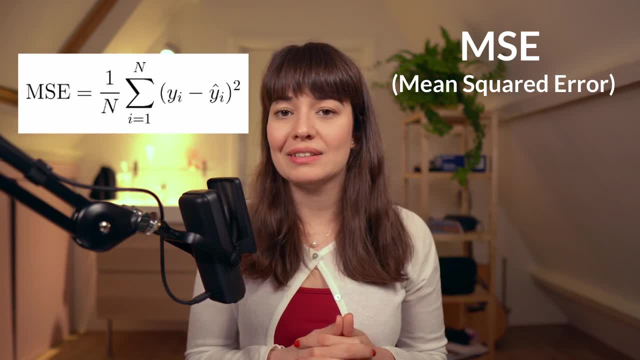 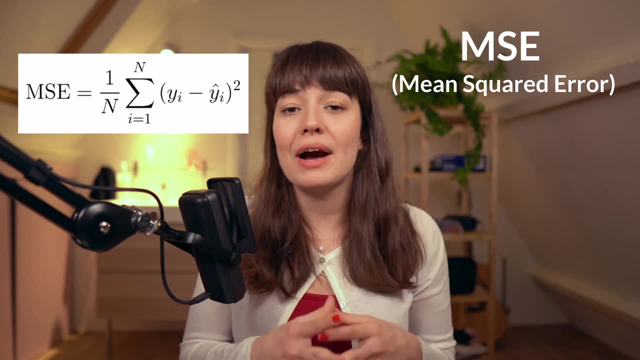 the square of all the errors and then taking their mean. By doing that, you are letting the greater error values to impact this mean squared error value And that's why you need to take all the more by exaggerating their importance, by getting their square. But this value, sometimes the mean. 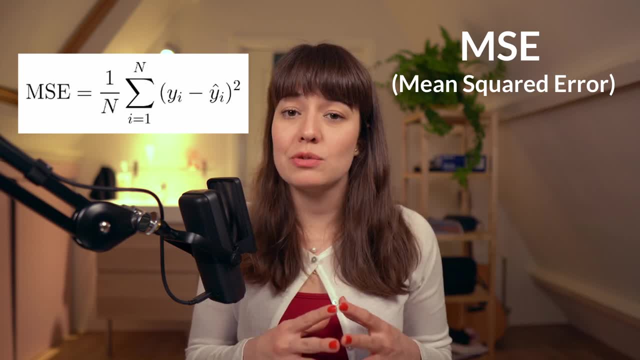 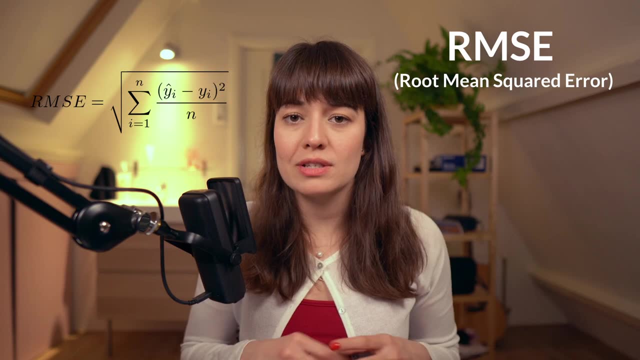 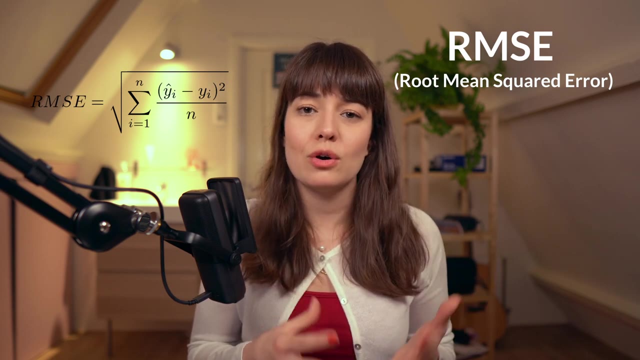 squared error value sometimes can be a bit hard to understand. That's why instead we use root mean, squared error, And that is calculated by again taking the square of all the errors, getting their mean and then getting the square root of this final value. So it's basically the square root of 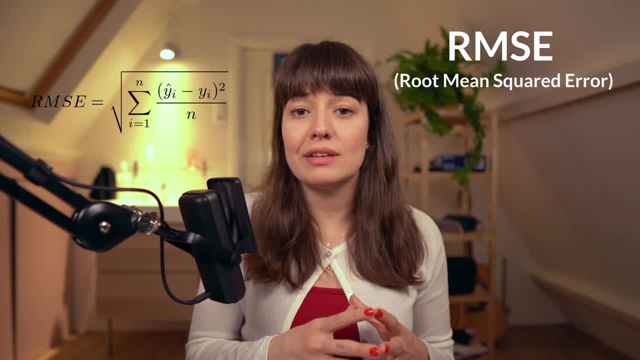 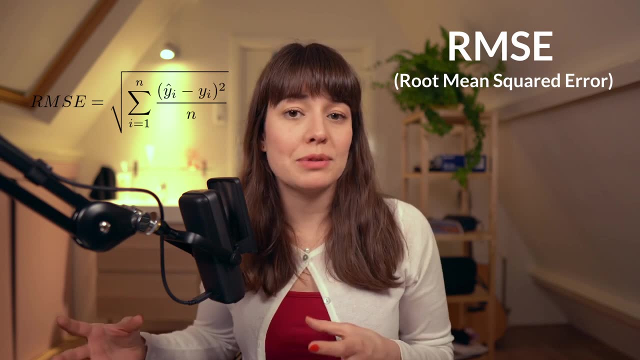 mean squared error. By doing that, you're still exaggerating the importance of the greater error values, but still you're bringing it down to the scale of mean absolute error metric, so that it's easier for you to compare these two metrics and understand what might be going wrong in your model. 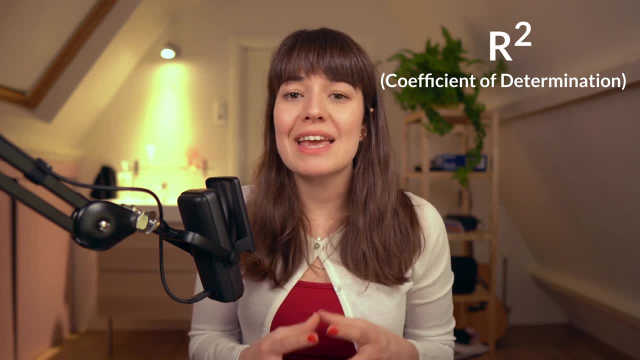 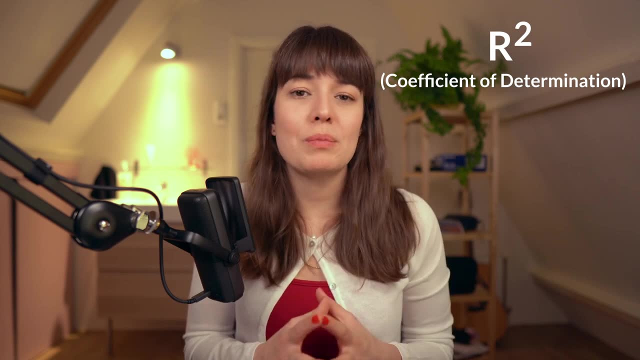 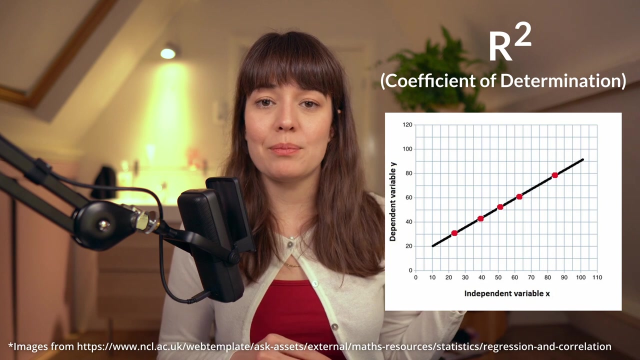 R squared, or coefficient of determination, gives us a good measure of how well your model fits this data. So it's basically the metric of how much the real values vary from the curve that your model came up with. So if you look at this example, 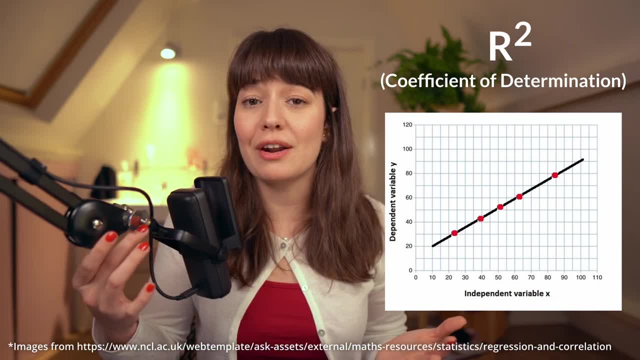 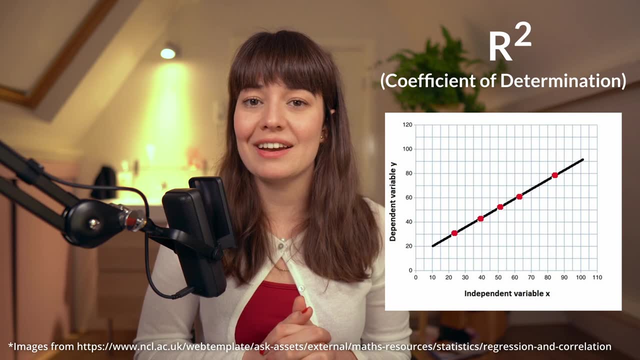 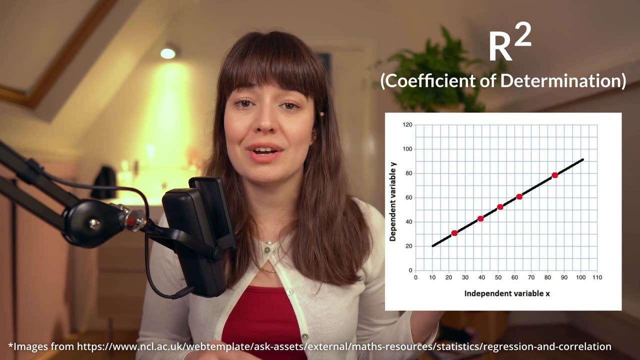 let's say, this line is the curve that our model came up with and the dots are the values of the real values of the instances that we have in our data. So if all the values lie perfectly on the curve that our model came up with, our R squared value is going to be one, Whereas if our model 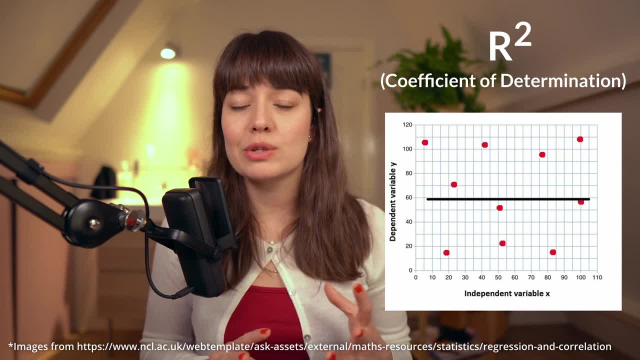 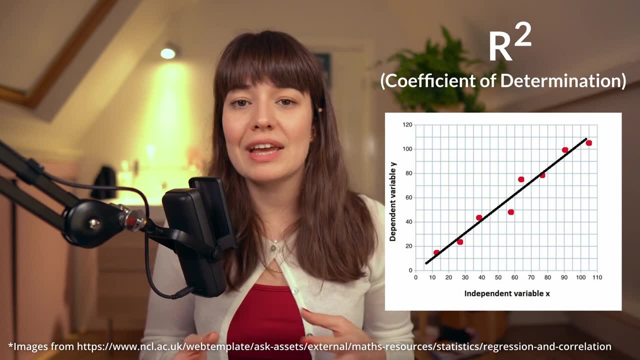 does not fit the data at all. our R squared value is going to be zero And for anything in between where our model is fitting a little bit better or a little bit worse, we're going to get a value between zero and one. So for R squared, the higher the value, the better. between zero and one.